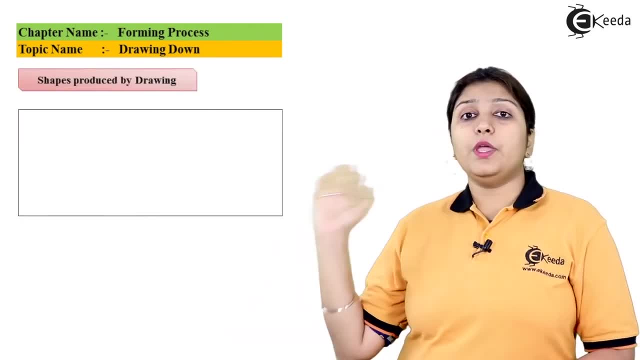 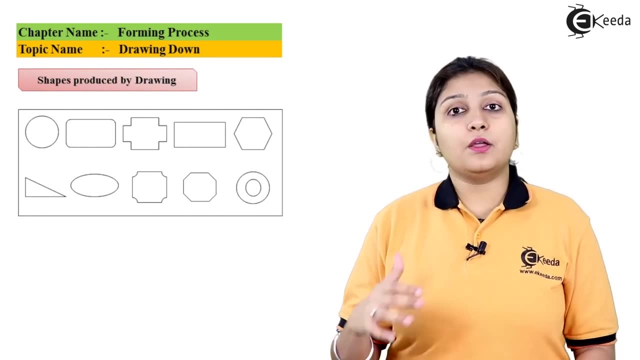 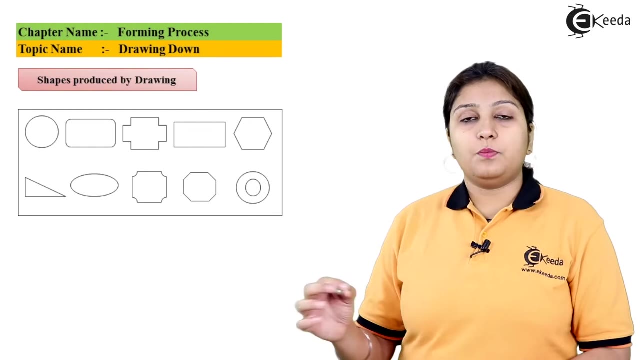 blooms, billets, etc. In this diagram you can see various shapes which are produced by drawing down process. So, as I have told you, only circular rods are not made. You can make rods or any other bloom or billet of different shape. Only the opening of that shape should be of the shape. 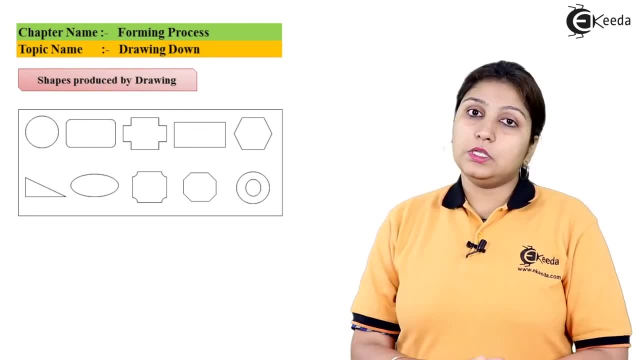 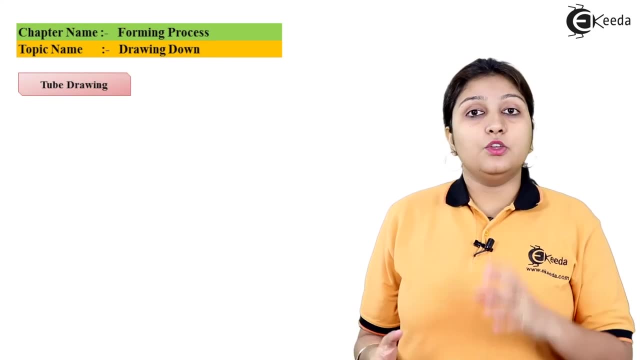 which is required. So in this way drawing down process takes place. Drawing down process can also be stated as tube drawing. So in tube drawing what happens is your section gets thinner, But as the name is tube, it is a circular section. So again it can be. 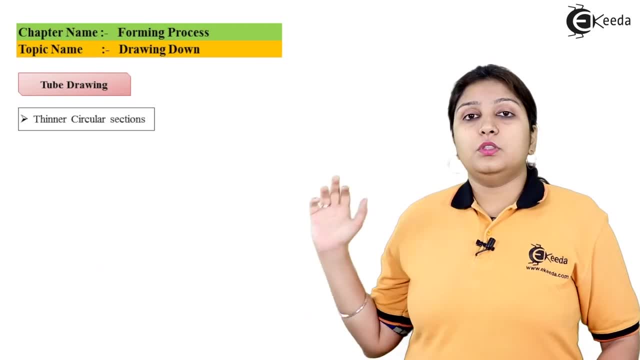 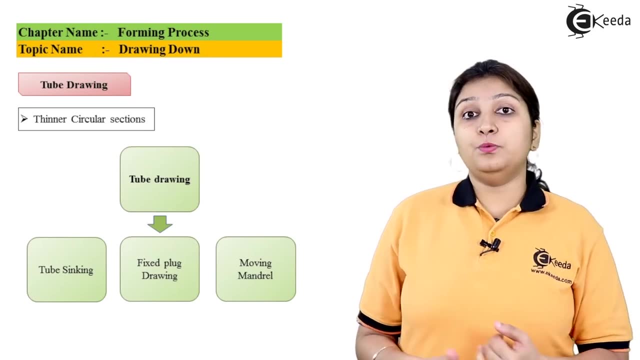 classified into various types which can be shown in our video. So these are the basic three types in which the tube is classified. So tube drawing can be classified as tube swinging, or your mantle can be used, or else a plug can be used. So we will see one by one all the three types. So we will see. 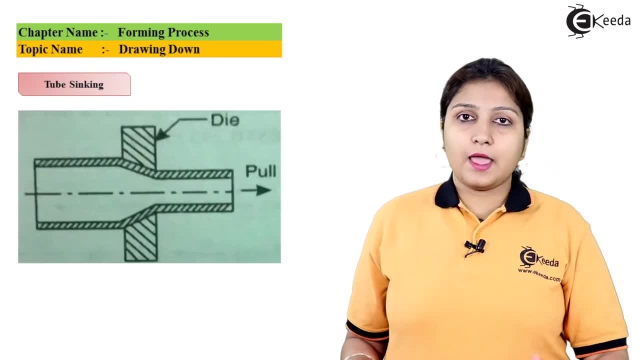 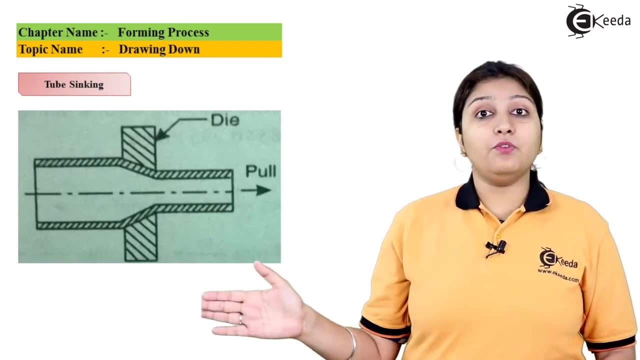 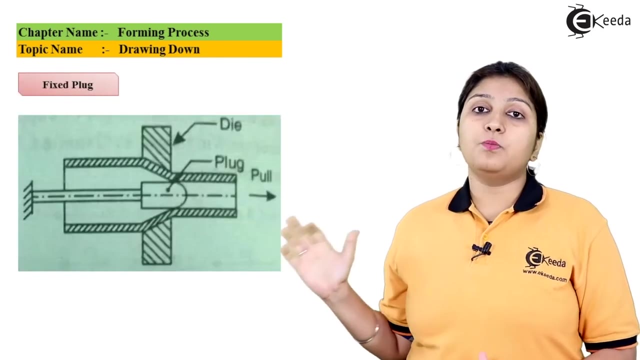 three types. So in this diagram you can see there is a single die which has the shape of the object to be made. Your object is passing through the die and it is moving in a forward direction. This is a general drawing process, which is your tube sinking process. This is a second drawing down process. 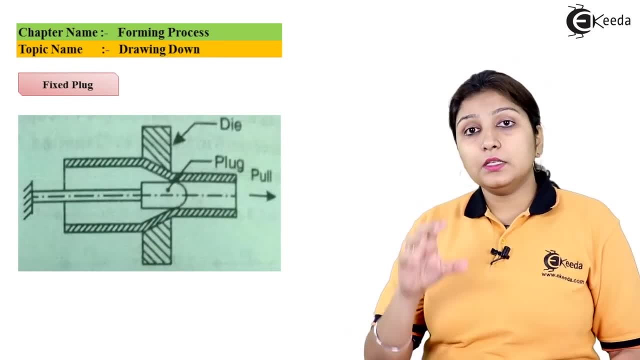 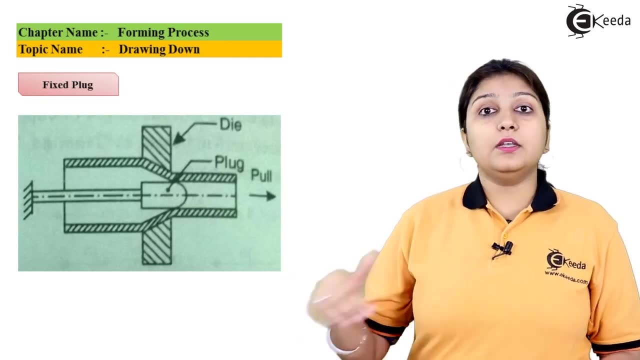 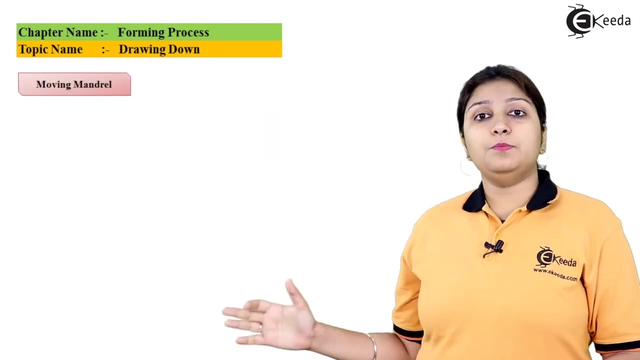 which is a fixed plug process. In this a plug is fixed at the entrance of your die. Material is passing but because of the plug the interior part of your material gets the shape of that plug. So this is a plug fixed process And the last part is your moving. 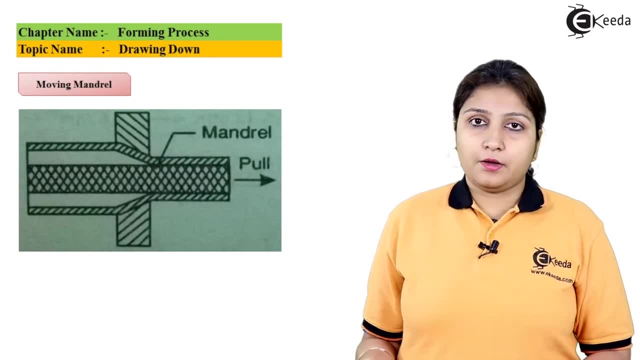 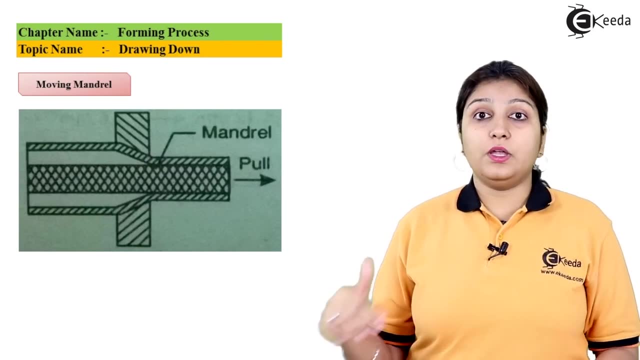 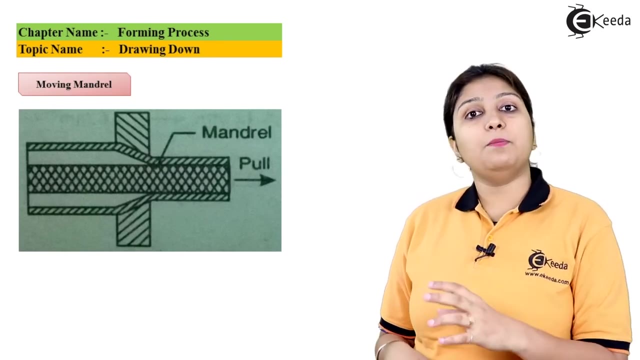 mandrel types. Instead of a plug, you are using a mandrel. So what happens? your mandrel is rotating and it also helps in giving the internal structure or your internal shape to your object. So mandrel is moving, It is passing continuously through the die and material is forced through. 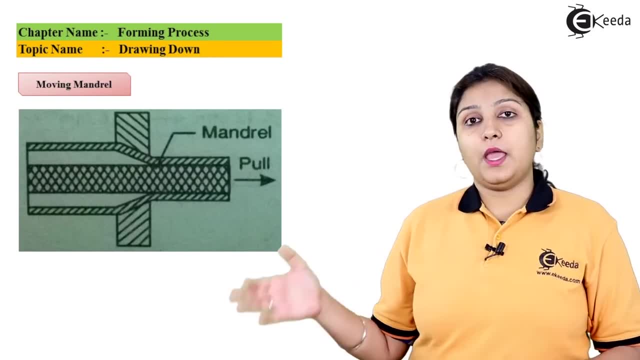 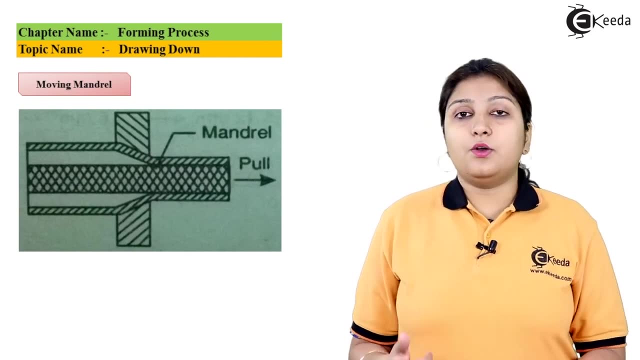 the mandrel, So a circular object can be made as your final product. So these are the three types of different tube drawing processes. So in this way, on a lump sum way, a drawing process is explained. Thank you for watching this video. Stay tuned with IKEDA and do subscribe our channel. 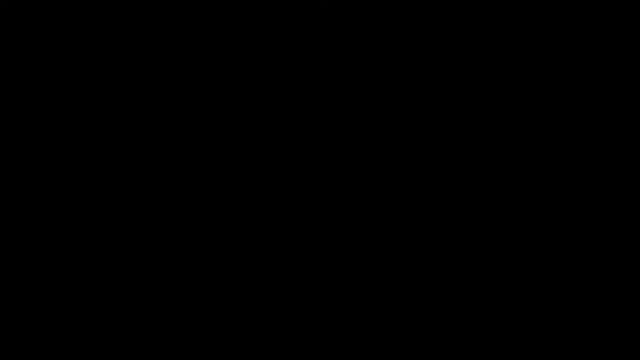 IKEDA Subtitles by the Amaraorg community.